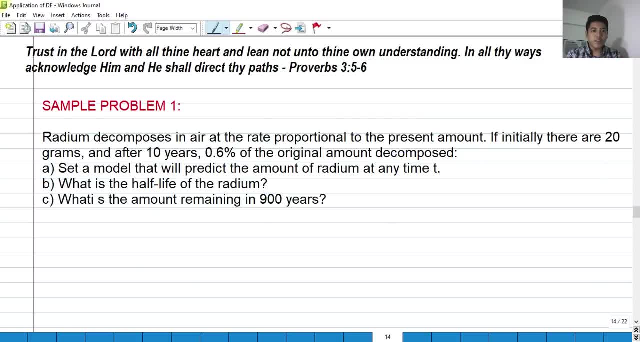 that will predict the amount of radium at any time t. so we are asked to have an equation that will predict the amount of radium at any given time, t. so in order for us to do that for letter a, okay, this is the problem. the very first thing you're going to do with the de always set up the equation just like. 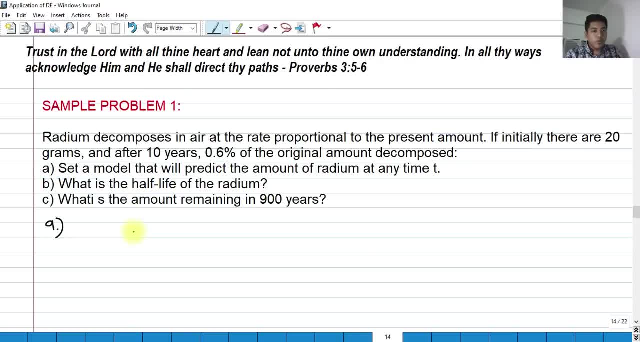 what we are doing in newton's law fully. so we have the right equation: dx over dt is equal to kx- okay. if we perform separation of variable, dx over x would now be equal to k- dt- okay. and if we integrate both sides of the equation, we'll be having: 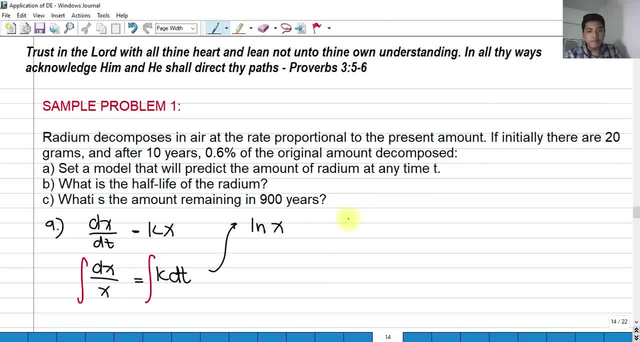 this: okay, dx over x is ln of n, x is equal to kt plus arbitrary constant c or the constant of integration c. so if we raise these two equation, both sides, if we exponentialize this, okay, so exponentiate. so we have e raised to l and x would simply be x and we have e raised to kt plus c, but by loss of exponent we have 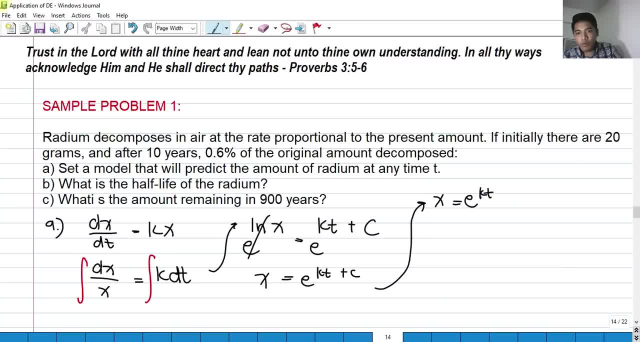 x is equal to e raised to kt, multiplied by e raised to c. but e raised to c is simply equal to c. so we have now our general solution a while ago. that we have. okay, i derive it for you, for you to understand, how did we arrive at that general solution? that is not the answer for letter a. 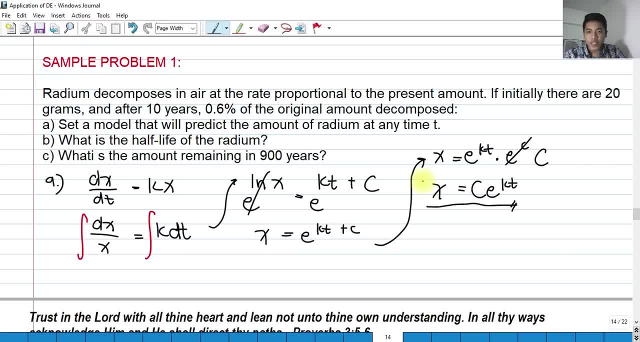 okay, as you can see here, xd is the amount of substance at any time, t. so if we plug in any values of t in this equation we could definitely get the x, given that we know the value of c and we know the value of k. so, just as like in our newton's law of pooling, we need first to determine the values of c and 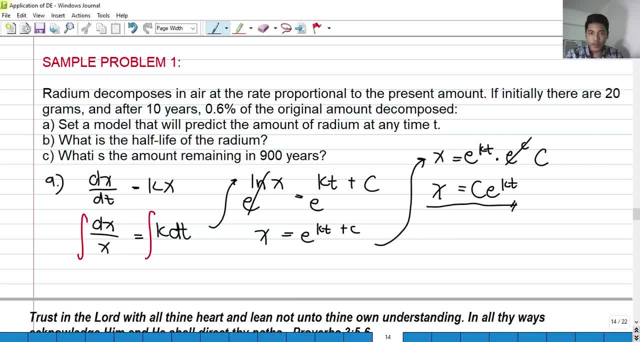 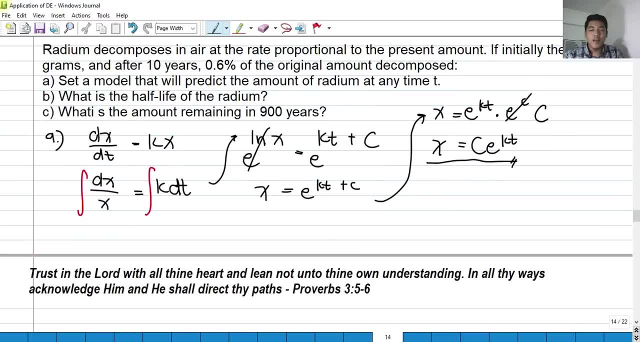 the values of k and arrive at a certain equation that would give us the amount of radium x at any time, t, so let's try to find the values of c and k. okay, so at time is equal to zero, okay, initially. okay, our value of x is 20 grams. that's what the problem says. okay, so we? 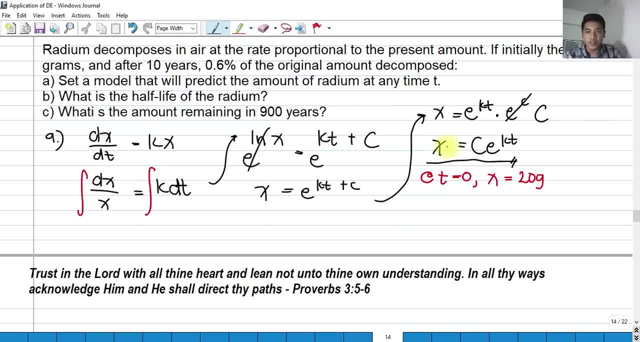 have. if initially there are 20 grams, that is times equals to 0, x is 20 grams. so if we're going to substitute this condition on our equation, we have: 20 is equal to c. e raised to k times zero- a times zero is zero. e raised to zero would become one. so definitely our answer for c is: c is equals to 20.. 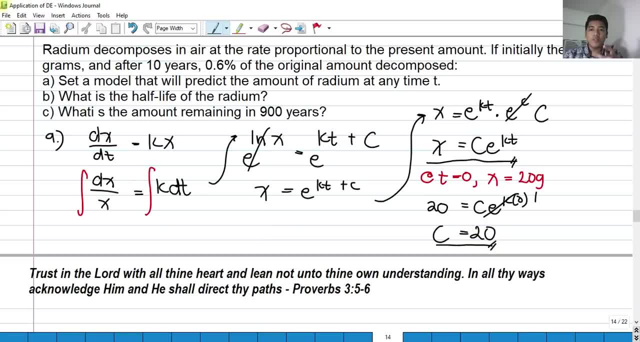 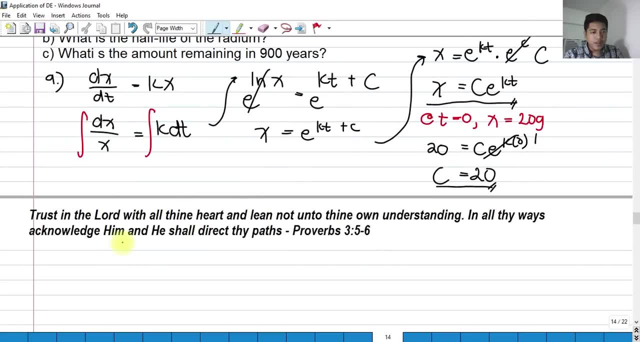 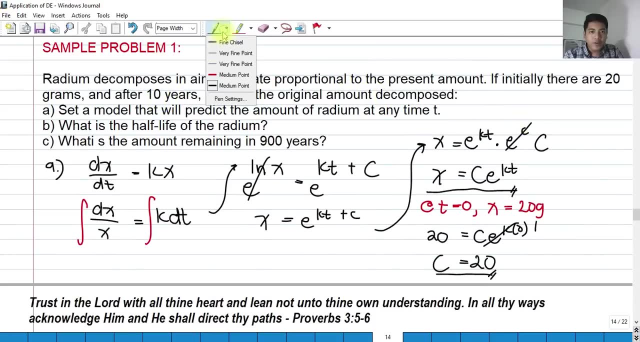 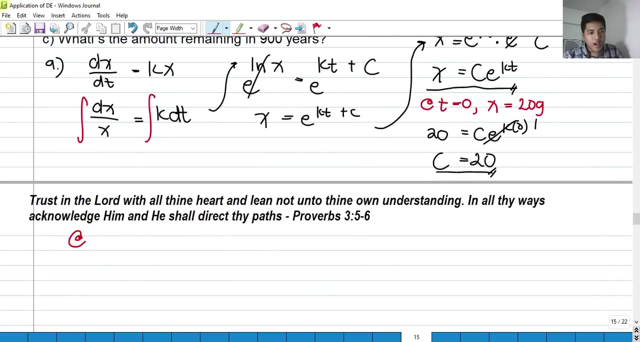 after we determine the value of c, it's now time to determine what is the value of k. okay, so if we determine the value of k, so we have the second condition, it tells us: okay, after 10 years, after 10 years, 0.6 of the original amount decomposed, so it means at time, is equals to 10 years. okay, 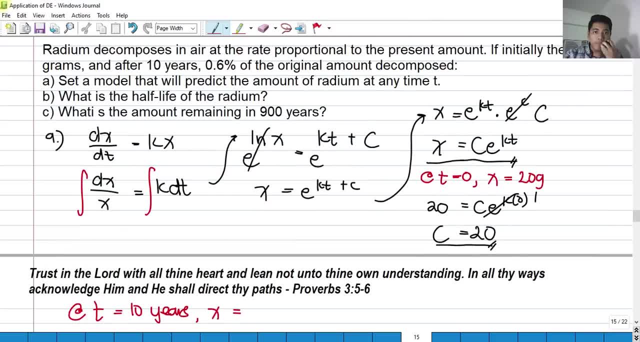 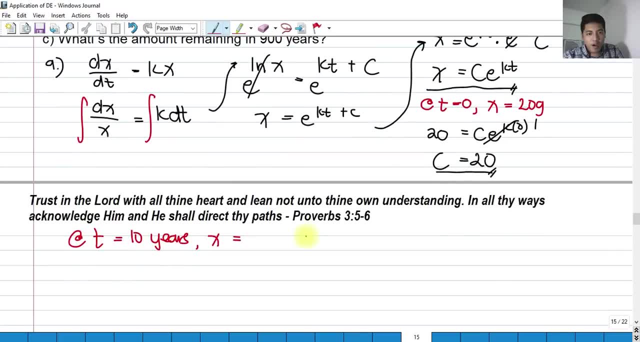 the value of x now would be reduced by 0.6 percent of the original amount. how do we compute that? the original amount is 20 minus okay, 20 multiplied by 0.6 percent is a percent. if we want to make it a decimal, so that we can multiply it by 20, that should be 0.006. we will be dividing 0.6 by 100. 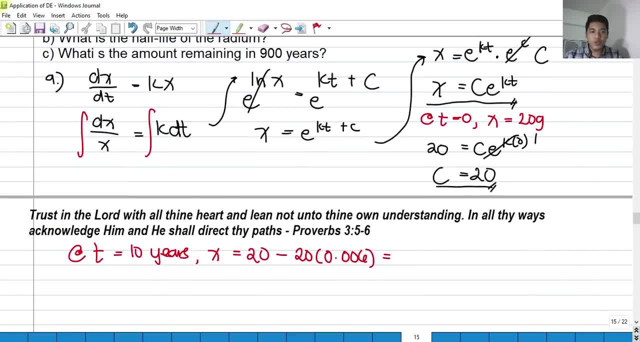 and if we're going to divide 0.6 by 100, we're going to divide 0.6 by 100, and if we're going to get the amount of radium, okay, after 10 years that should be 19.88. okay, 19.88 grams. so this would be. 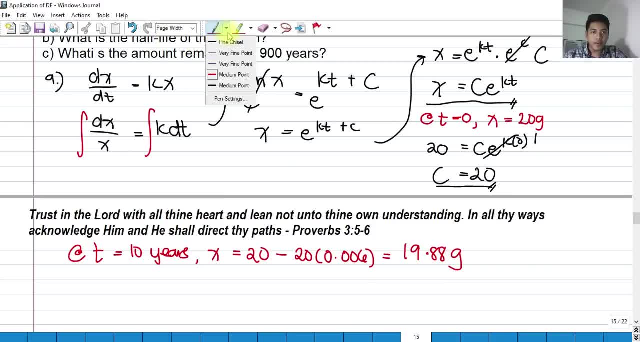 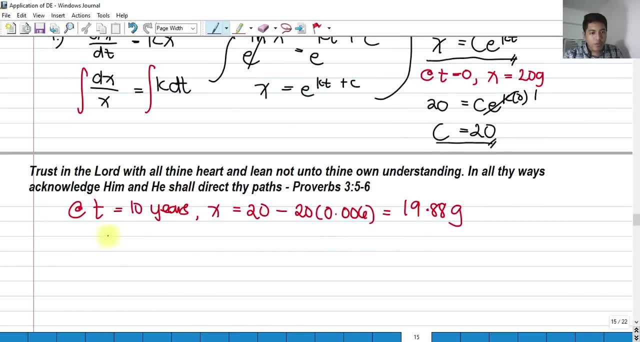 the amount of radium after 10 years. okay, so back to our equation. we have- uh, we simply substitute. our equation is c, e raised to kt. but we know the value of c is u times the juicy. so because we think along theance line, okay, we have to have 19.88 to 9.88, or if you use 0.18 that will be 13, because we have 19.88. now we already know n equal is equal to 1. accessory, which is the c. a while ago, e raised to k, multiplied by which is 10. okay, so we have now: 19.88 is equal to 20, e raised to 10p. okay, by algebra we need to find k. so 19.88 divide both sides by 20. we have e raised to 10 k and if i m going to take this k, i will fill this together. and this is the value for x, because we will find k in this section. 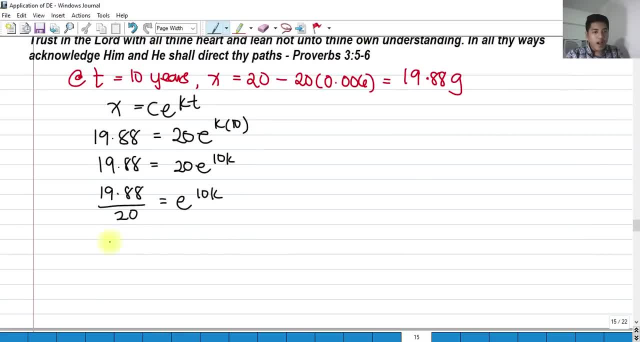 The natural logarithm of both sides of our equation we have: ln of 19.88 over 20 is equal now to ln e raised to 10k. okay, So this would cancel. definitely ln of e would cancel. We are left with, on the right side of the equation: 10k is equal to ln 19.88 over 20.. 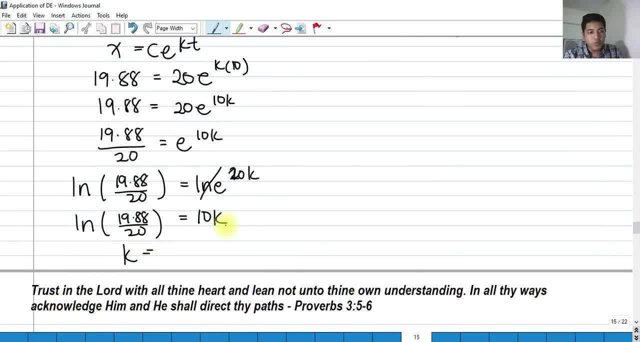 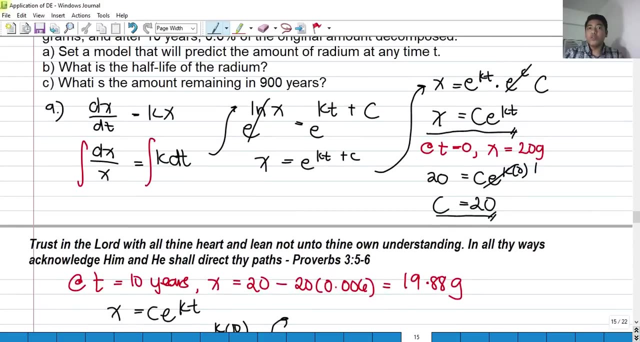 And to get k, simply we have: k is equal to 1 over 10, ln of 19.88 over 20.. And now we have our answer for letter a, a modal equation that would compute the amount of remaining radium at any time t. 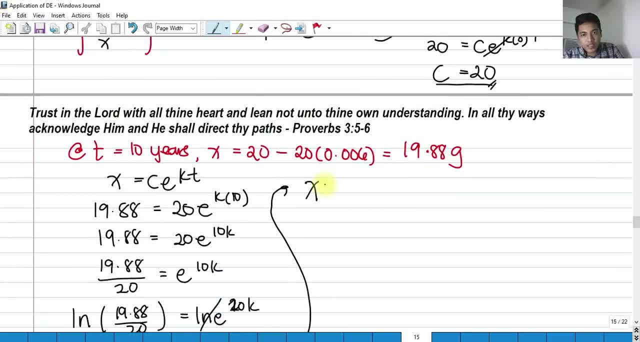 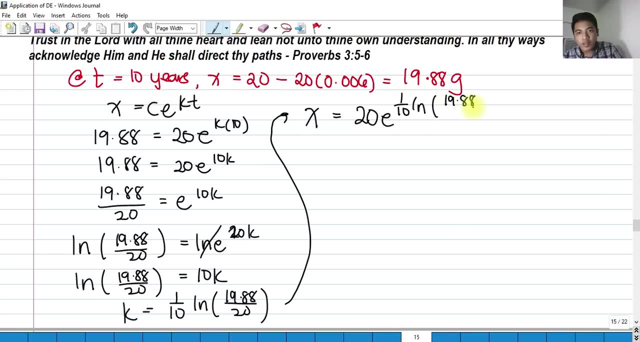 So, going back, so our answer would be: x is equal to c, e, k, t. Our value of c is 20.. e Multiplied by k. what is our k? That is 1 over 10, ln of 19.88 over 20 multiplied by t. 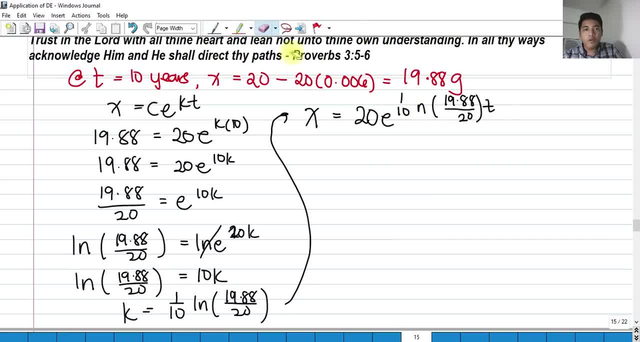 So this is our answer for our first question. letter a: a modal that would give the amount of substance at any time, t See if we are going to substitute any values of t here. since we know the c and k, we can. 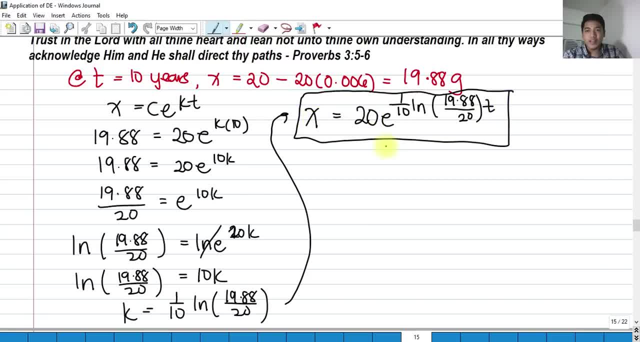 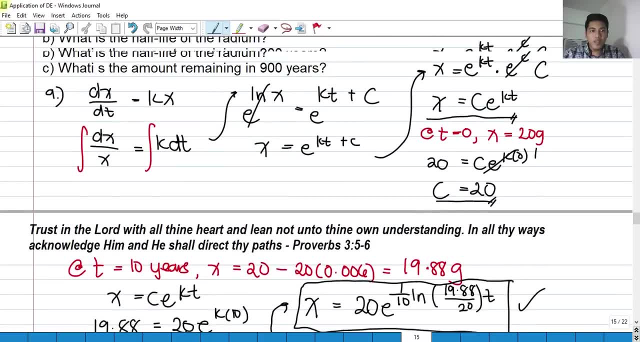 arrive always At a certain value, x. So that is the answer for our letter a. But for letter b let's try to solve. Okay, Letter b: what is the half-life of the radium When we say- let me rephrase the question- 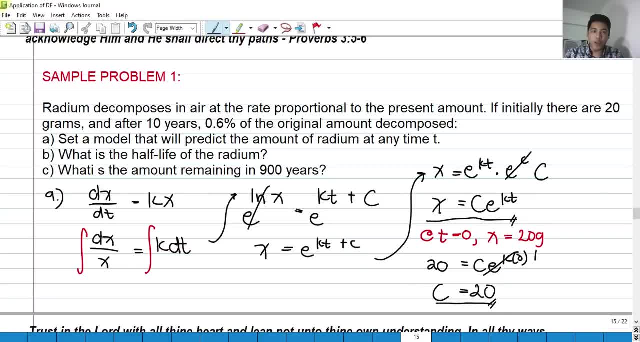 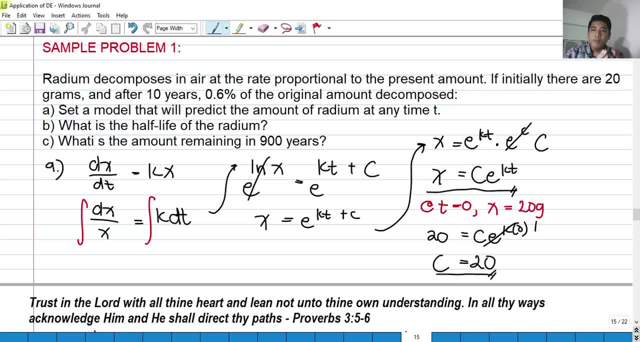 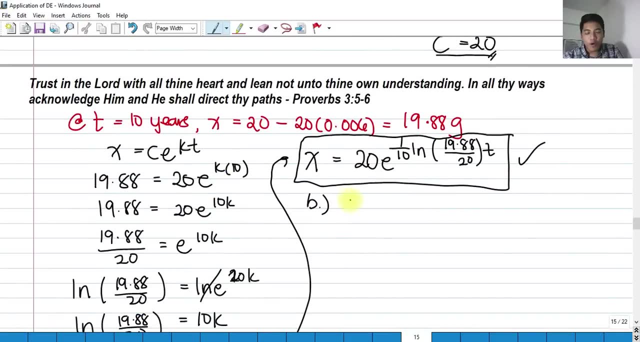 When will the radium be half-life? Okay, When? Okay, The half-life of any amount is the we are going to divide by 2. The initial Amount. So if initially we have 20 grams, the half-life of 20 grams is 10 grams. 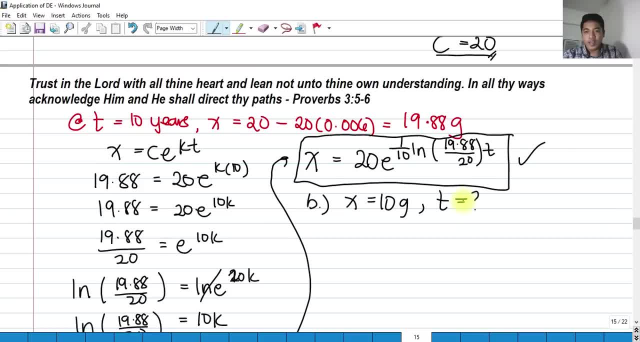 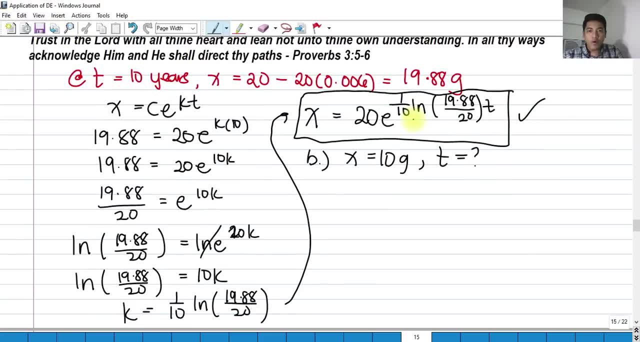 Okay, We are asked: what is the time it takes for 10 grams okay to decompose? So plugging it into our equation. this is our model equation. It is important always to get the model equation. Okay, This is our model equation. 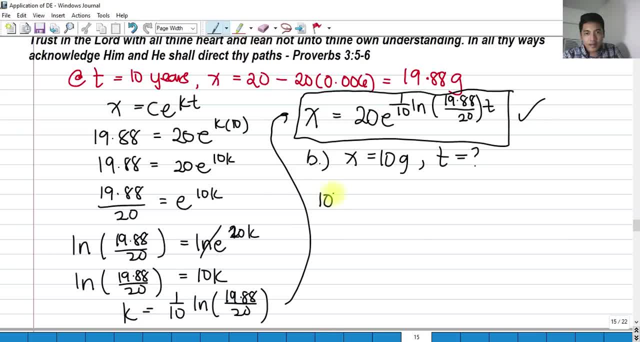 Plugging it in our model equation, We have 10.. Okay, 10 grams, This is equal to 20, e 1 over 10, ln of 19.88 over 20 multiplied by t. Okay, And we need to solve for t. 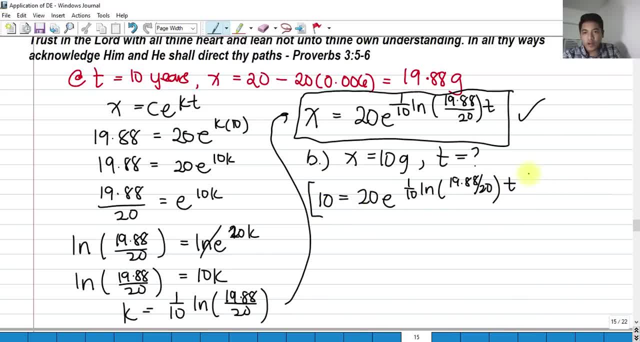 But before we do that, if I'm going to divide both sides, okay, the question is when? Okay, When will be the radium have a half-life? Okay, That is the question. So, if I'm going to divide this both sides by, 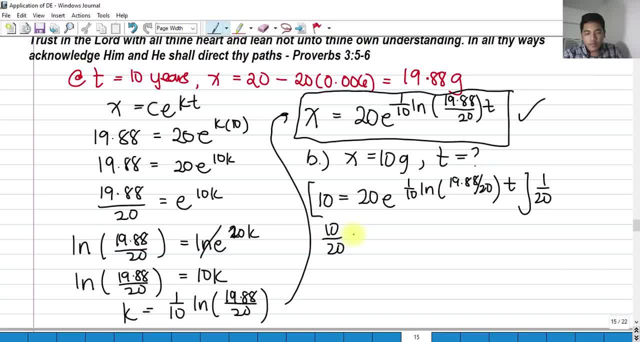 So we have 10 over 20 here and we have by properties: okay, this T is multiplied to the whole expression K, So I can rewrite this as T over 10, okay, or 10 or T times 1 over 10. ln of 19.88 over 20, okay. 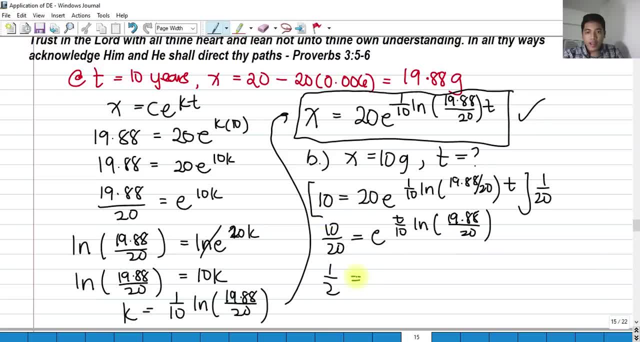 So 10 over 20 is 1 half and by properties of natural logarithm I can put this as the exponent of the ln. So we have E raised to ln 19.88 over 20, T over 10.. 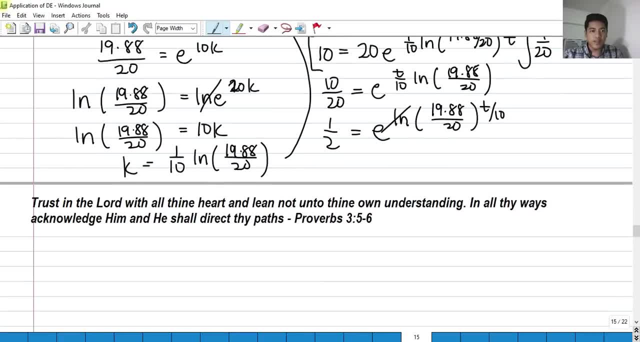 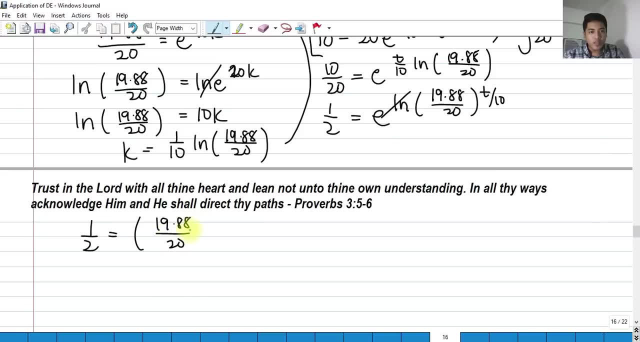 So we can cancel out E raised to ln. that's right. So we are left with: 1 half is equal to 19.88 over 20, T over Raised to T over 10, and we need to solve for T. 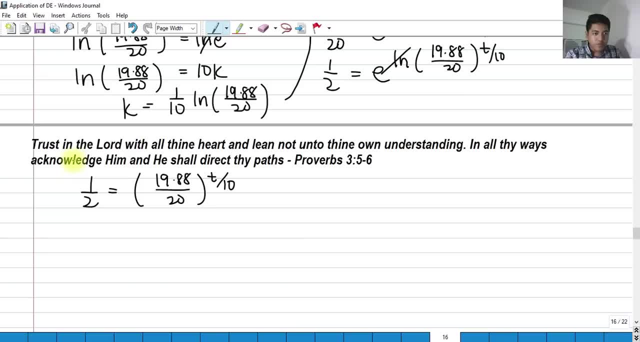 And if we're going to get the natural logarithm of both sides of the equation, so we have ln of 1 half ln of this By properties of natural logarithm. I can put this exponent again before the ln: okay. So we have T over 10, ln now of 19.88 over 20, okay. 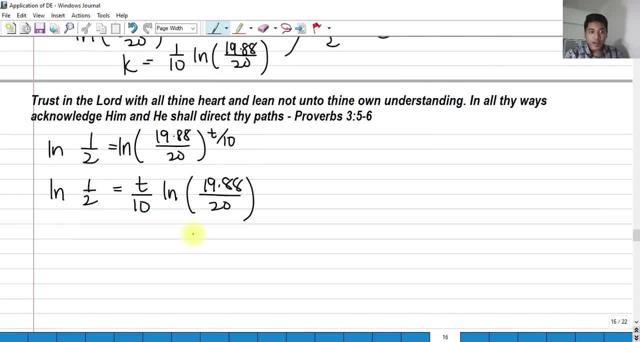 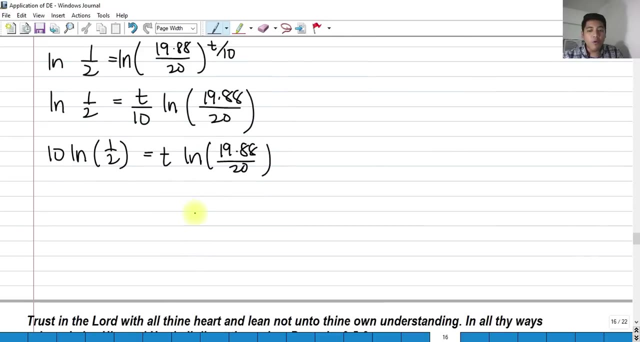 And we can. So we can now solve for T. okay, If we multiply this both sides by 10, we have 10 ln of 1, half is equal to T ln of 19.88 over 20,. okay, So we can solve now for letter T, because that is the time it takes for the radium to have the half-life, which is 10 grams. 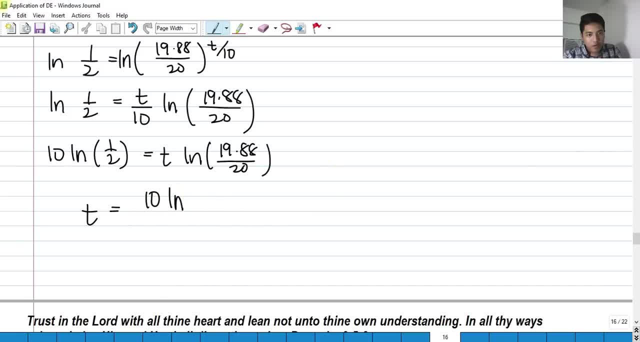 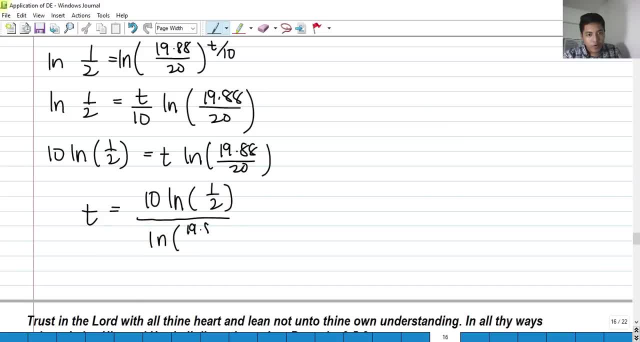 Over ln of 19.88 over 20.. So if we're going to evaluate that with our calculator, let's try 10 ln of 0.5, or 1 half ln of divided by ln of 19.88 over 20,. 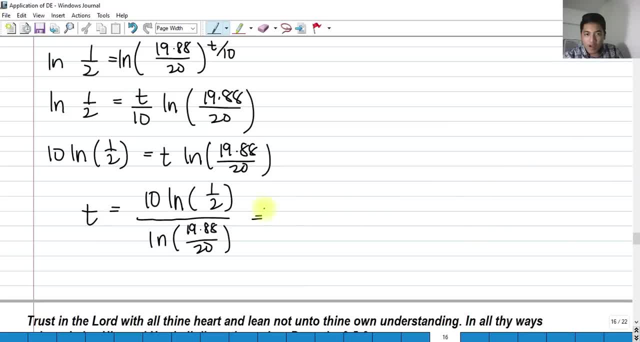 the time it takes is for it to have a 10 gram okay Substance. that is 1,151.. The unit of time is years. okay, At least for this problem. okay, At least for this problem. So that is our answer. 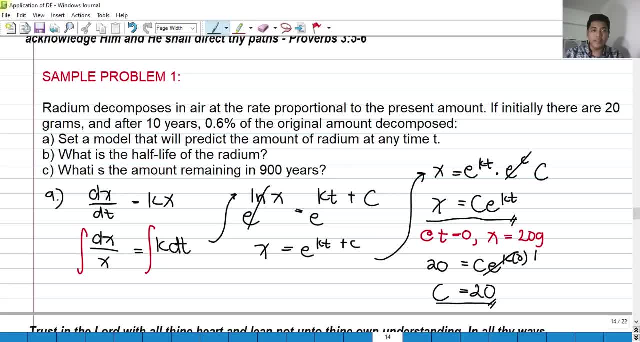 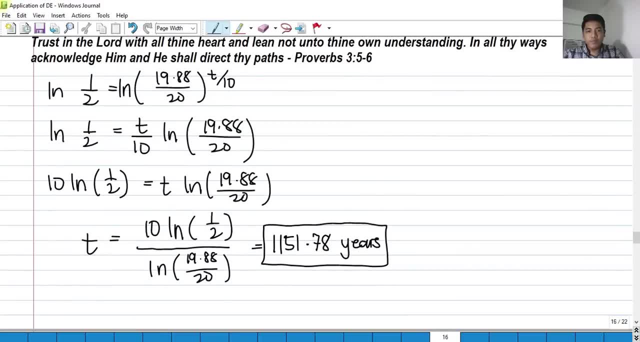 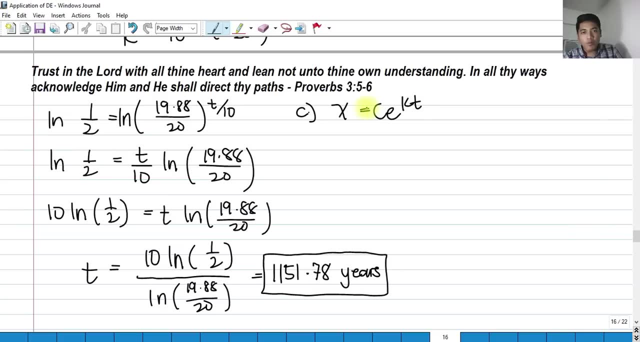 When will it reach its half-life? Okay, when? Okay, Number three: what is the amount remaining in 900 years? Okay, this is very pretty obvious. okay, We have now our model equation a while ago and our model equation is X. 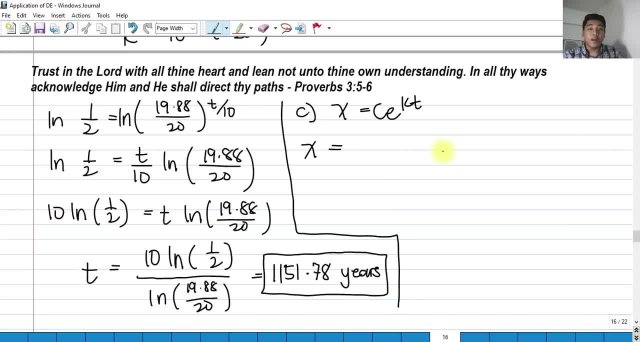 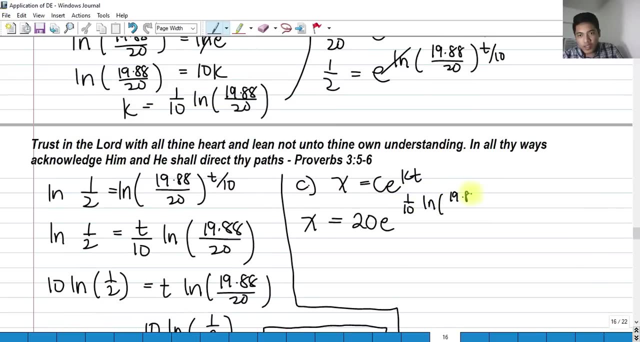 What would be the amount remaining after 900 years? Imagine so we have our C is 20,, E raised to what is our K, again, K is 1 over 10,. okay, ln of 19.88 over 20, multiplied by T. 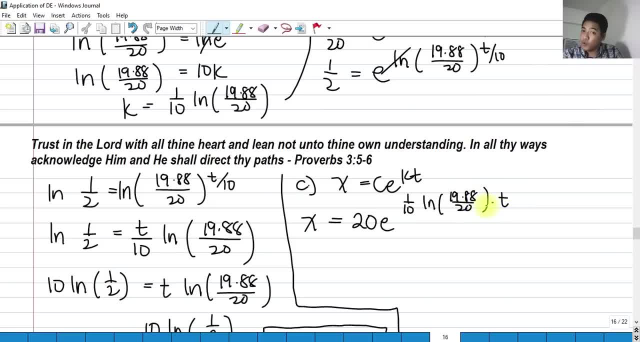 Take note that T is not inside the ln. it is multiplied by T, okay. So in other words, if I'm going to do this, 20, E raised to T over 10, ln of 19.88 over 20,, okay. 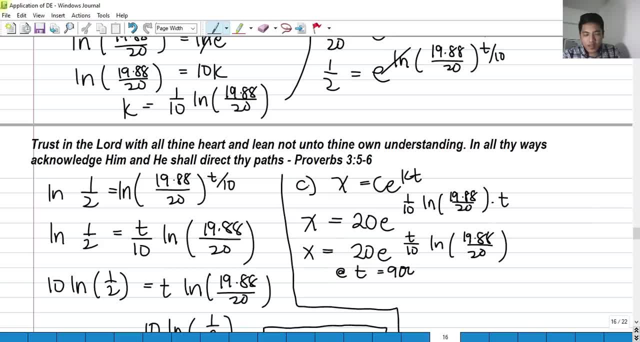 Plugging it at time is equals to 900,. okay, So we have. X is equals to 20, E, okay, Raised to 900, because that's our time: 900 years over 10, ln of 19.88 over 20.. 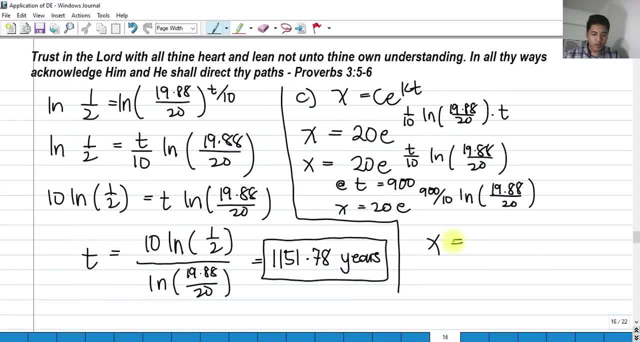 And our answer should be: if we input this- let me just calculate it- So we have 900 over 10, ln of 19.88 over 20, our answer should be what? 11.63.. Now, what is this 11.63?? 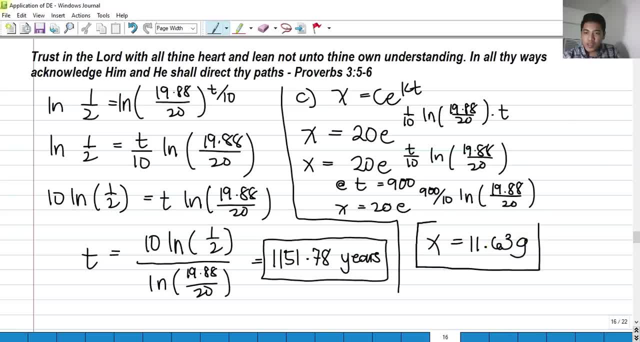 That should be in terms of grams, because initially the given is in terms of grams, So we expect that what we get is also in terms of grams. So that would be the amount remaining ratio after 900 years. Okay, let's try another problem. 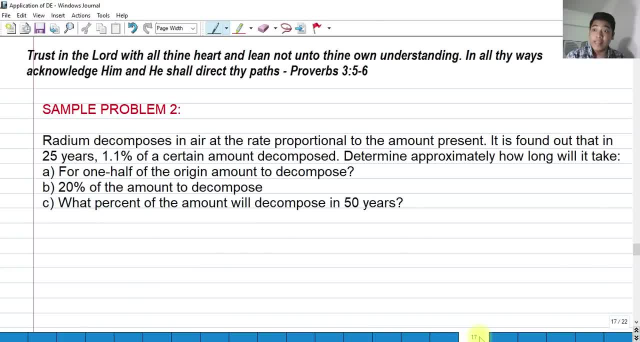 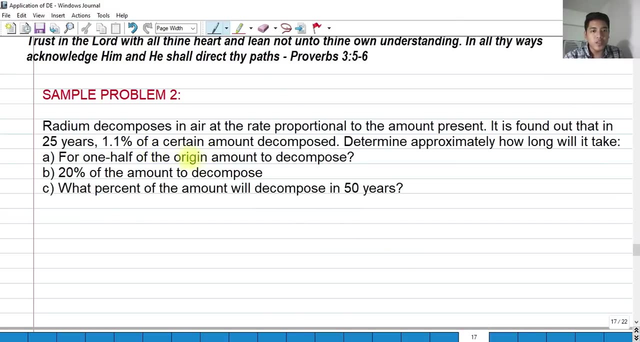 So for this problem, again it's a problem involving a decay of certain element. So again, radium decomposes in air at the rate proportional to the amount present. It is found out that in 25 years, 1.1 certain okay of a certain amount is decomposed. 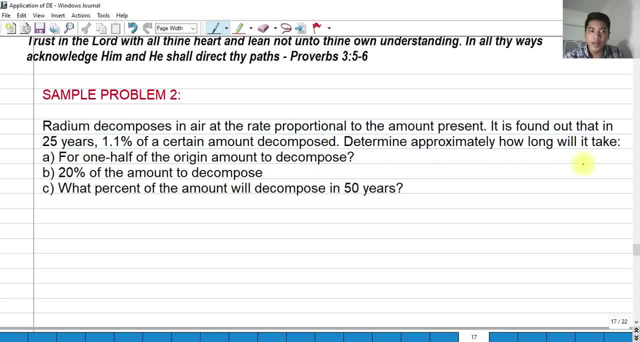 Determine approximately how long will it take for one half of the original amount. okay, this is the original amount. okay, original amount to decompose. okay, There is a great difference between our problem a while ago and in this problem, As you can see here. okay, the amount of present. okay, is not initially given. okay, 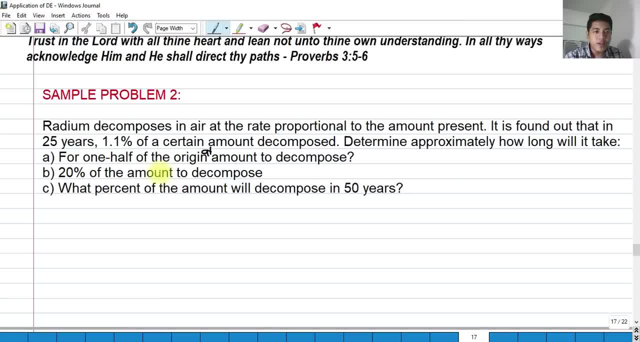 So it only says that after 25 years, Okay. Okay, After 25 years, 1.1 percent of a certain amount is decomposed. But initially the problem does not give us any initial x, okay, So if we are not given any initial x, it is safe always to assume okay. 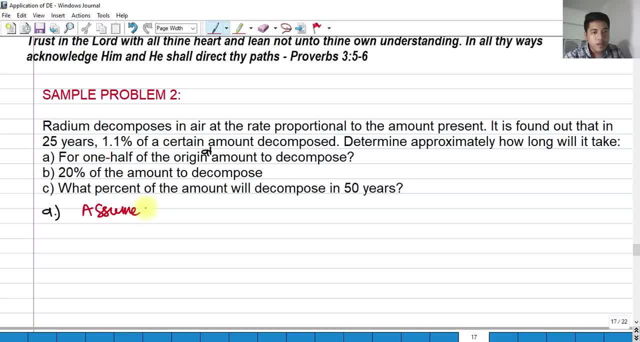 let's say, assume x is equals to 100 grams. okay, Whether it be for population or substance, let's assume 100 grams. okay. So, but if it is given, you should use what is given. okay, But if it's not, it's convenient to use 100 because we are dealing with percentage. okay, always. 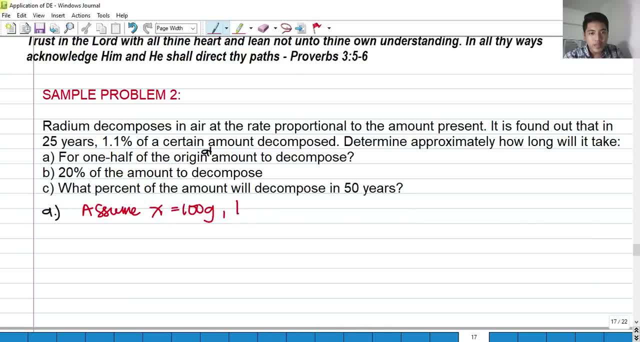 So assume that x is 100 grams. at times equals to 0. That's the initial amount of the radium. You can also use 50.. You can also use 20 grams, Okay, But 100 grams is much easier because we are dealing with percentage okay. 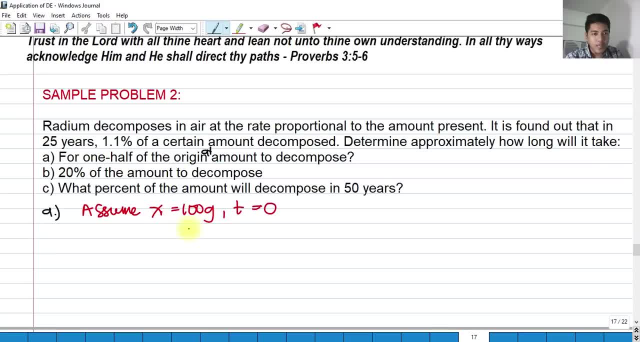 So assume that we have 100 grams at times equals to 0.. Our model equation or our equation general equation is this: okay, I've derived this a while ago, So we need to find C again, okay, First, we need always to come up with a model equation, even if it is not asking the problem. 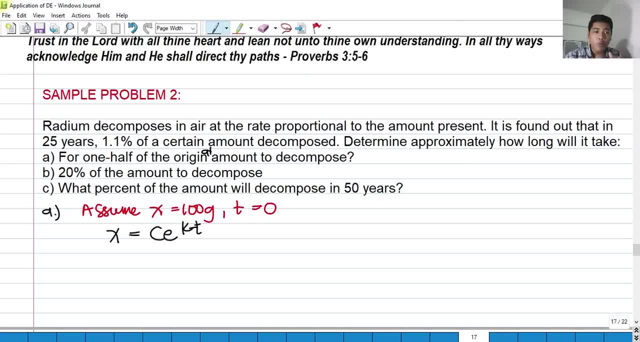 So that you would be able to solve for what is being asked in the problem. So we need to find C and we need to find K. So initially we have: 100 is equal to CE multiplied by E raised to K times 0.. 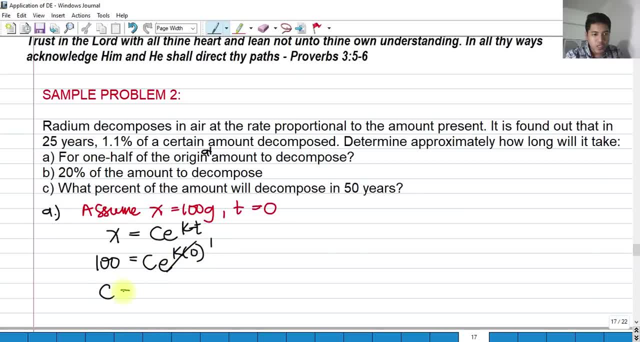 So this is K times 0. This is equal to 1.. So C is our 100, okay. So another condition to solve for K. It says it is found out that in 25 years at time is equals to 25 years. okay. 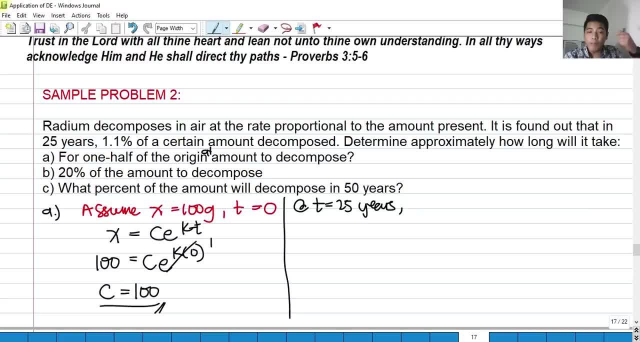 the amount is decomposed by 1.1%. Okay, The amount is decomposed by 1.1%. So if 1.1%, we have 100 grams minus 1.1 grams, because the 1.1% of 100 is 1.1.. 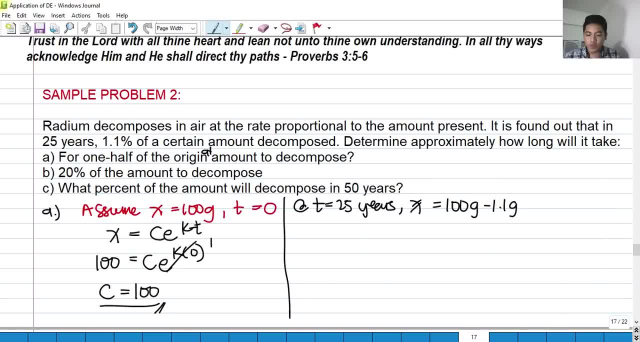 So definitely, if we do that, 100 minus 1.1, that is 98.9 grams. So that's why I chose 100, as I assume 100 grams, because it is easier to compute. okay, just like what we did here. 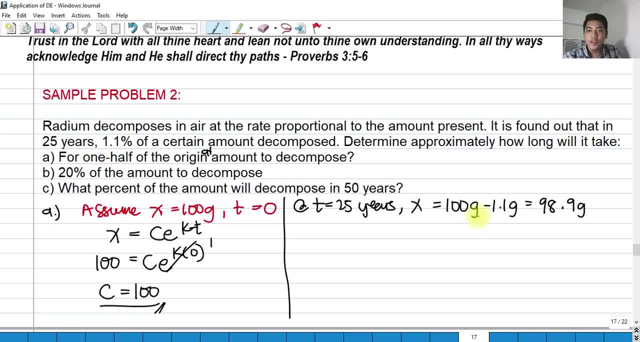 So again, after 25 years, the original substance decreased by 1.1%, and the 1.1% of 100 grams is 1.1 grams, so that we subtract 1.1 from 100.. So we have 98.9 grams. 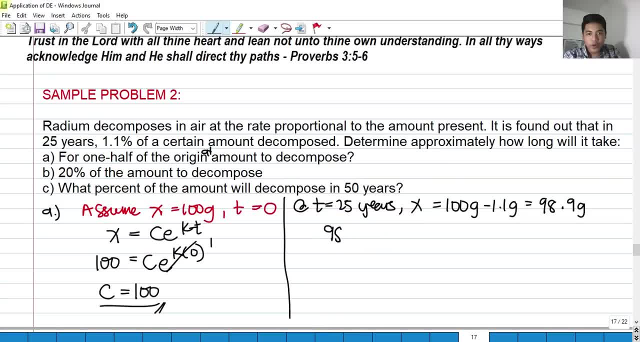 So again, our condition, we have 98.9.. That is the value now of our X after 25 years, is now equal to the value of C, which is 100, E raised to K multiplied by 25, because that is 25 years. 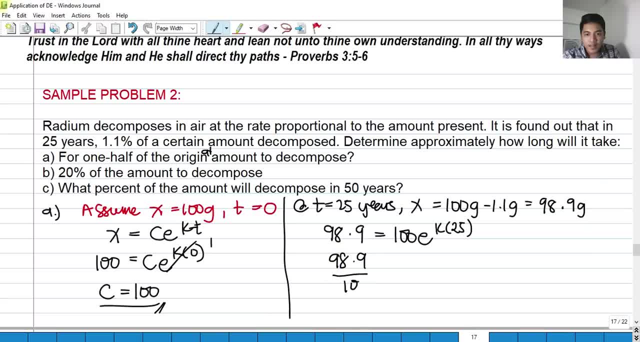 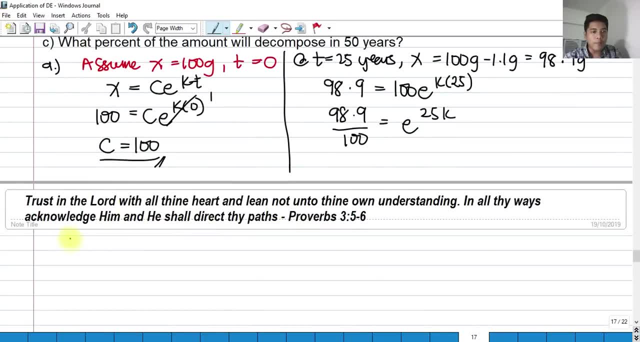 By algebra we have 98.9 over 100 multiplied by E, raised to 25K. And if we get the Ln of both sides, we know what will happen: Ln of 98.9 over 100.. 100 is equal now to LnE25K raised to 25K. 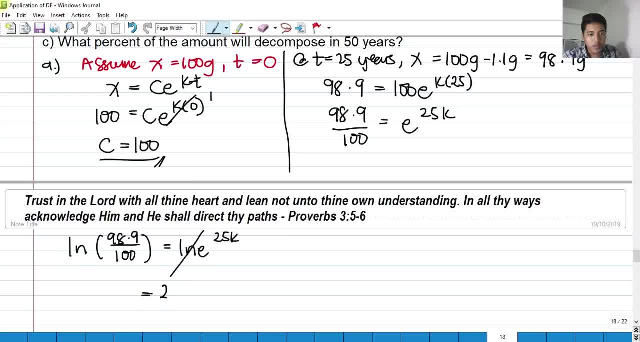 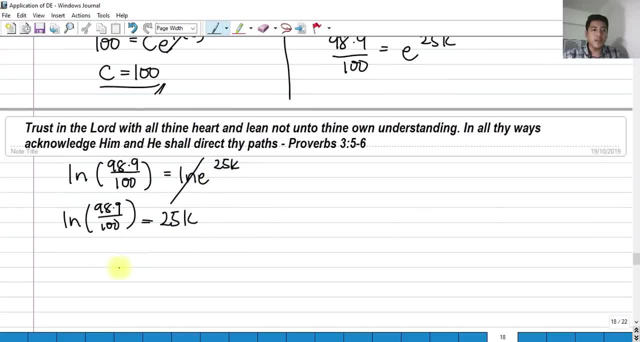 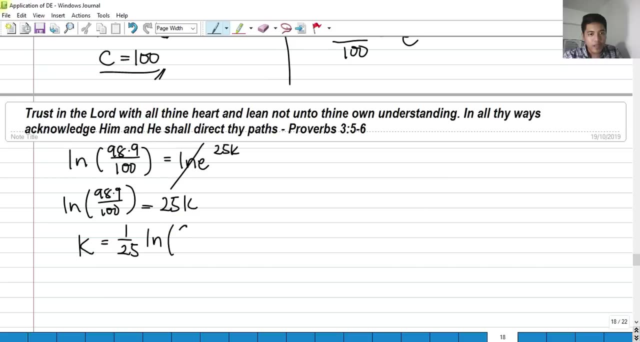 We have now Ln of E canceled, So we are left with 25K here and we have Ln of 98.9 over 100 here In order for us to get K we have. K is now equal to 1 over 25, Ln of 98.9 over 100. 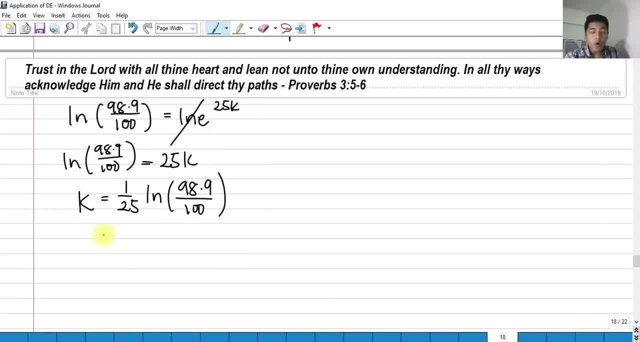 So that should be our equation. So our model equation now will be: X is equal to the amount of substance X at any time T should be. X is equal to the value of C is 100 multiplied by E, raised to 1 over 25 Ln of 98.9 over 100 multiplied by T. 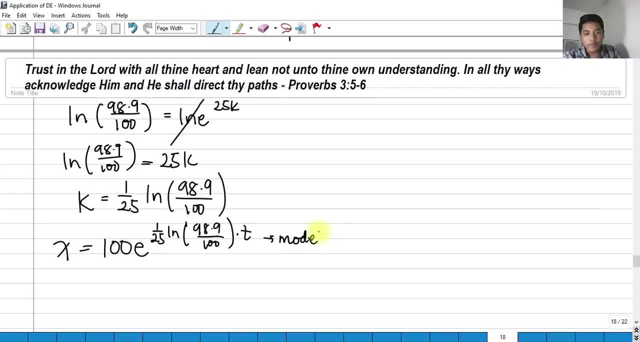 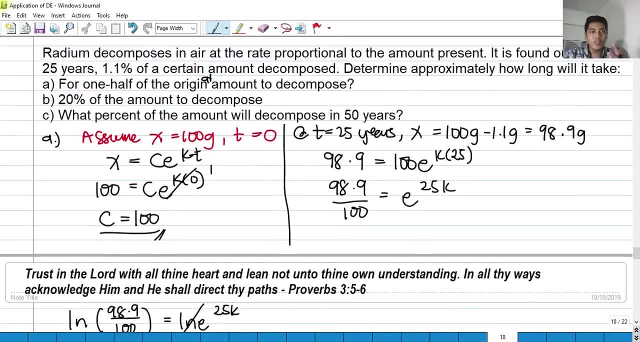 This is our model equation And therefore, if we get the model equation, if we know the value of C and K, we can therefore now answer what is being asked in the problem. So, for how long will it take this one? 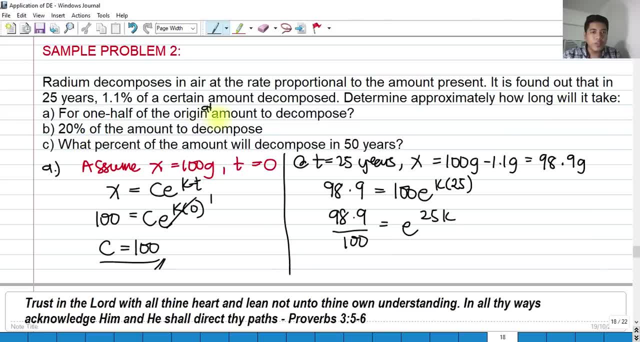 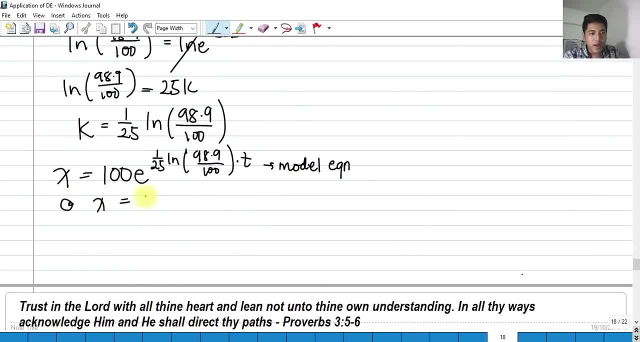 how long will it take for one half of the original amount to decompose? So one half of the amount. So it means at X is equal to one half of 100, this is 50.. What is our time, Okay? 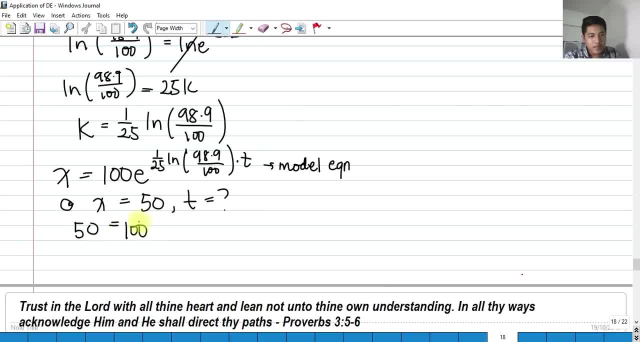 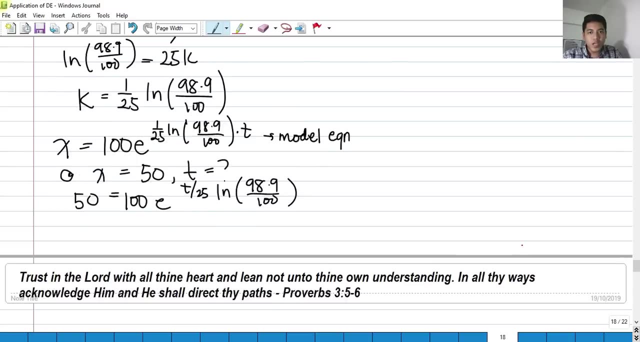 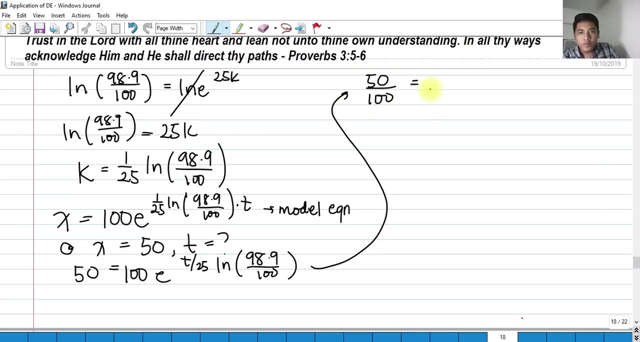 So what will happen? We have: 50 is equal to 100. E Okay, I can multiply this onto this. So we have T over 25 Ln of 98.9 over 100. Okay, And if I'm going to divide both sides by 100, we have now 50 over 100 is equal to. 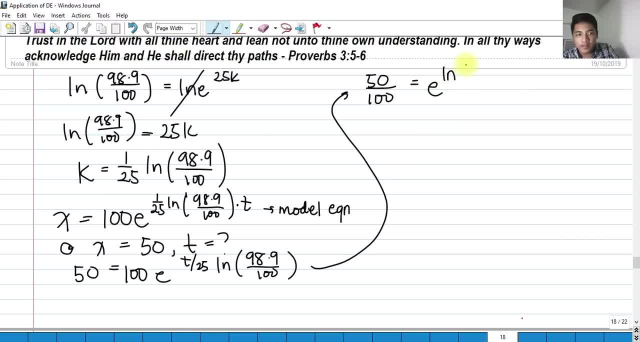 by loss of natural logarithm. we have Ln. I can have this as my exponent. So we have E raised to Ln. 98.9 over 100.. Okay, T over 25.. And I can cancel out E raised to Ln. 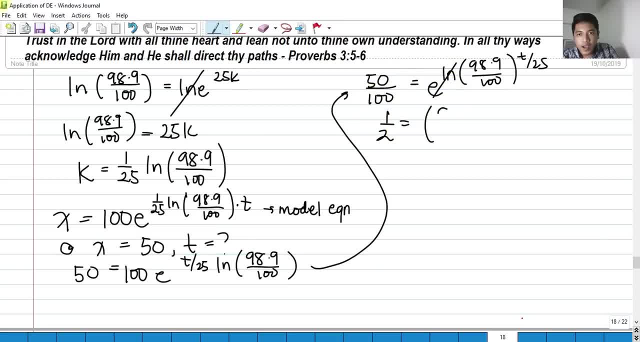 50 over 100 is one half, So we have 98.9 over 100 raised to T over 25.. So if I'm going to get the natural logarithm of both sides of the equation, okay: Ln of 98.9 over 100, T raised to 25.. 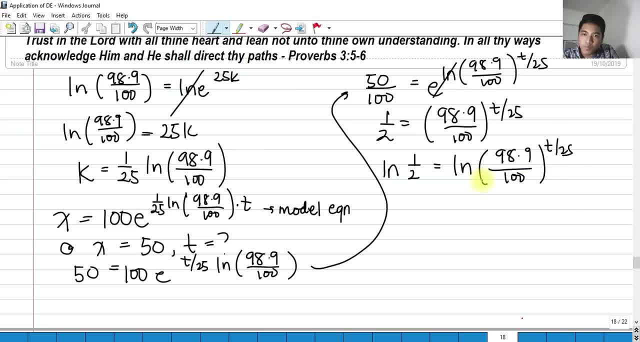 By properties of Ln. I can put this exponent before the Ln, So we have Ln raised to one half, So T over 25, Ln of 98.9 over 100.. Okay, And I can get T, So T would now be 25 Ln of one half over Ln of 98.9 over 100. 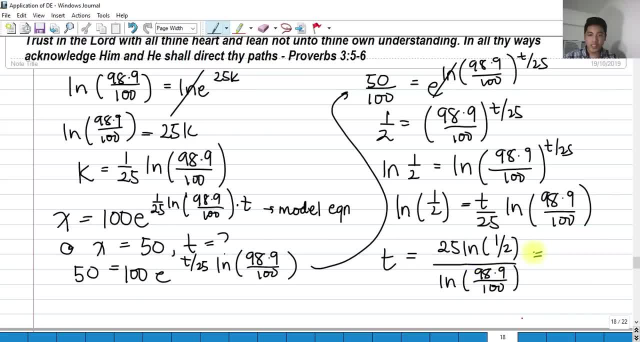 And the value of T should always be positive, because there is no such thing as negative time. Okay, So let me just calculate this Better, if you have your calculator with you, So the time it takes for it to achieve its half-life, or half of the original amount. 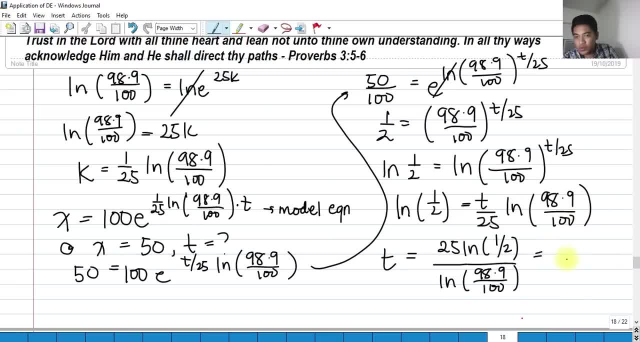 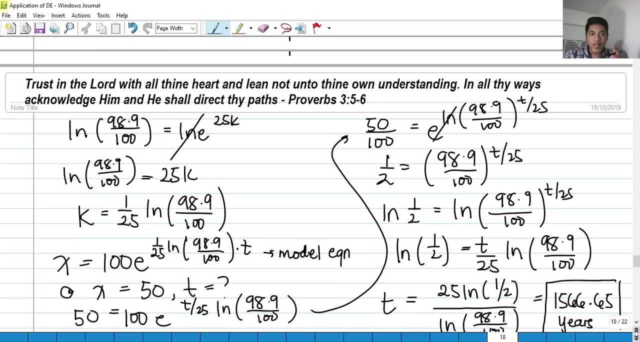 which we assume to be 100.. So that should be after 1,566.2.. Okay, So that's about 1.65,. again, years, because the unit that we're going to talk about here, or talking about here initially even, is in terms of years. 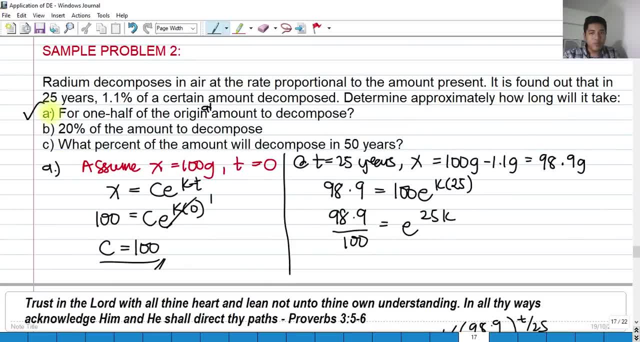 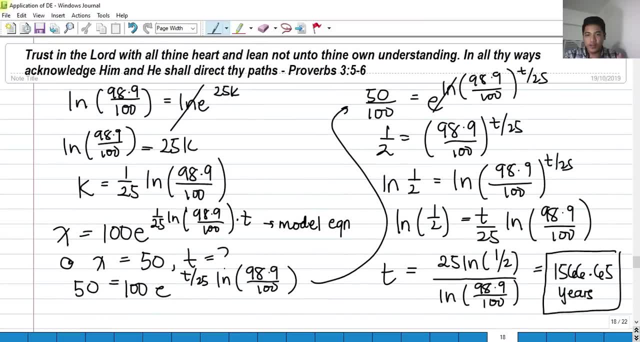 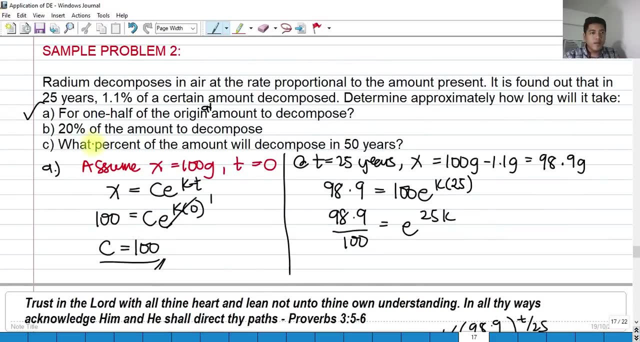 So that is our answer for letter A. Approximately how long will it take? It would take 1,566.65 years, Okay. So for letter B, determine approximately how long will it take? Okay, 20% of the amount to decompose. 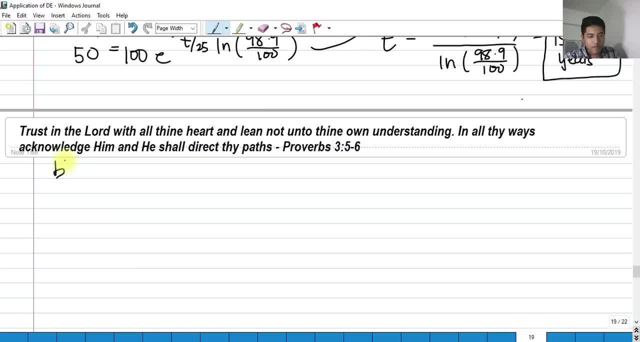 So 20% of the amount to decompose. If I have 100 grams, the 20% of 100 grams is 20 grams. So we are talking about 80 grams here because it decomposed 20%, So our X should be 80 grams. 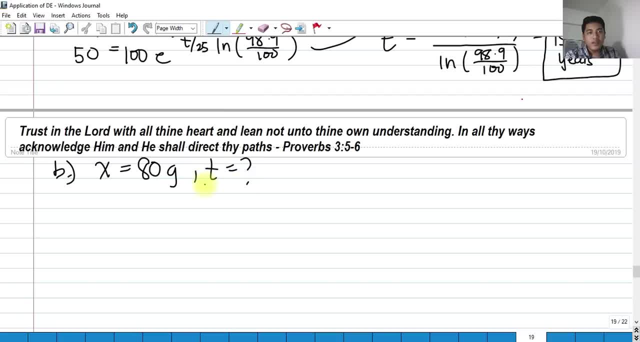 Okay, So what is the time for it to reach 80 grams? So, given in our model equation again, our model equation would now be: X again is 100, E raised to 1 over 25, Ln of 98.9 over 100 multiplied by T. 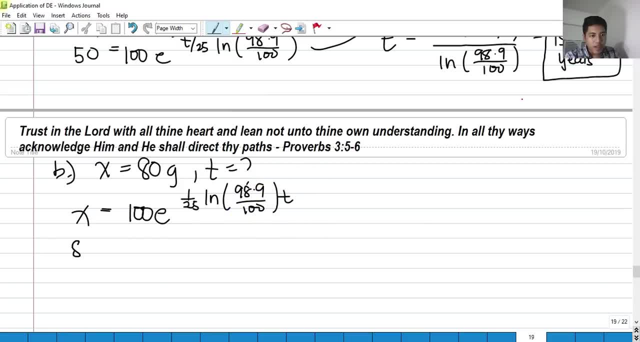 We need to solve for again for T. So we have: 80 is equals to 100 because X is our 80.. Okay Again, E raised to Ln of 98.9.. Okay, 98.9 over 100, T over 25.. 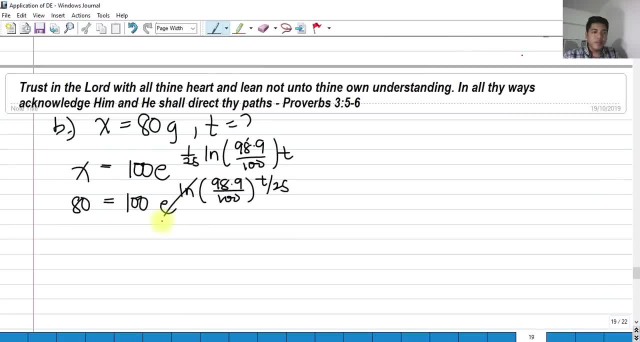 That's what we did a while ago. This would cancel, And dividing both sides by 100, I have 80 over 100.. Okay Is equal now to 98.9 over 100, T raised to T over 25.. 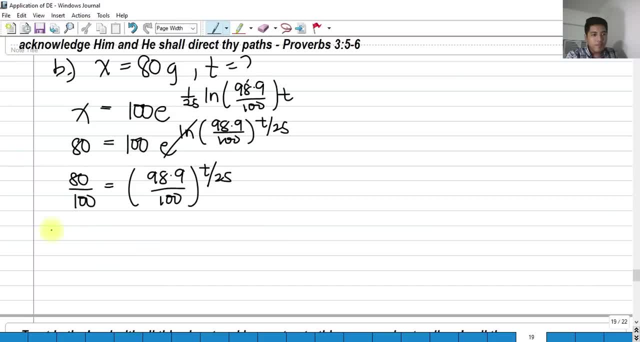 If I'm going to simplify this, okay, or get the Ln of both sides, what is this? Four-fifths, Okay, The lowest term of this is four-fifths. So we have Ln also of 98.9 over 100, raised to T over 25.. 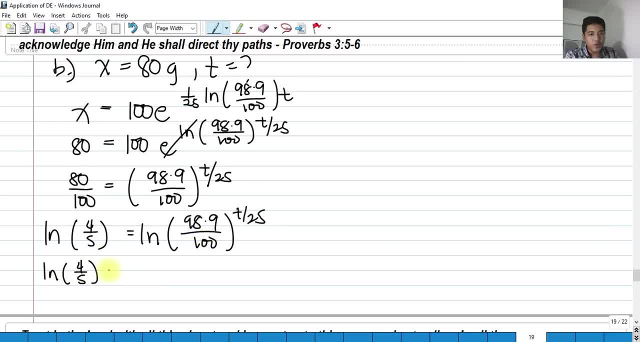 So by properties of Ln, I can rewrite the right side of the equation as T over 25, Ln of 98.9 over 100.. So if I'm going to furthermore solve for T, okay, because that is what is being asked. 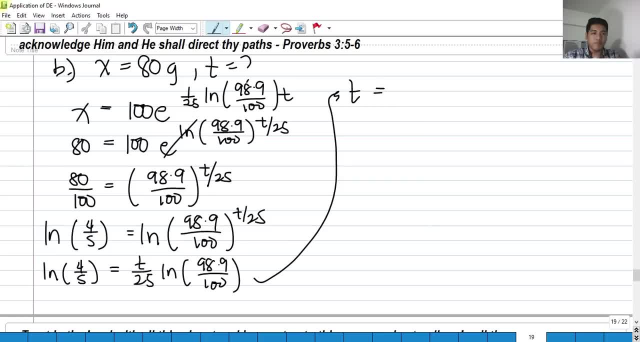 the time. okay for the radium to have 80 grams okay remaining. So we have 25 Ln of 4 over 5 over Ln of 98.9 over 100.. Okay, Let me solve this: 25 Ln of 4 over 5 divided by Ln of 98.9 over 100. 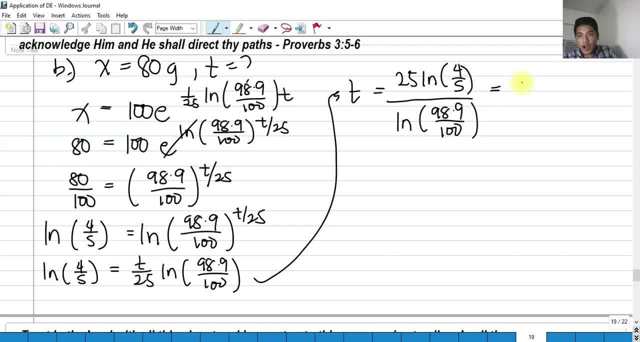 So we have an answer of 504.35 years. Okay, This should be our answer. After 504, approximately 504.35 years, the value of the radium would now be 80 grams. Okay, And lastly, let us go for letter C. 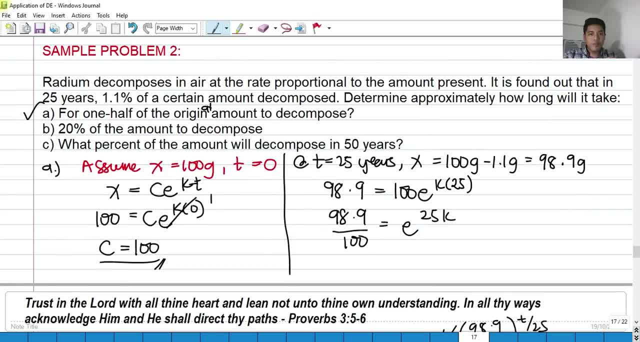 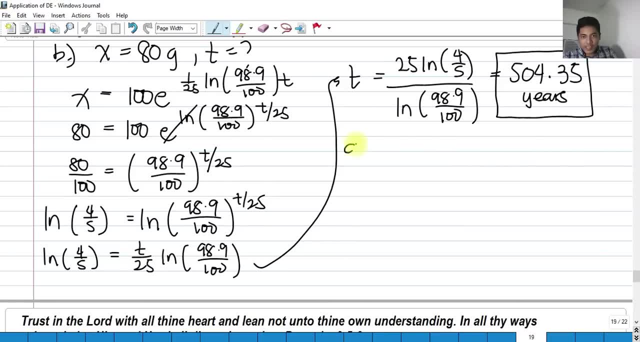 What is being asked for? letter C? What percent of the amount will decompose in 50 years? So what percent of the amount will decompose? Okay, He is not asking what will be the amount after 50 years, but rather what is the percentage. 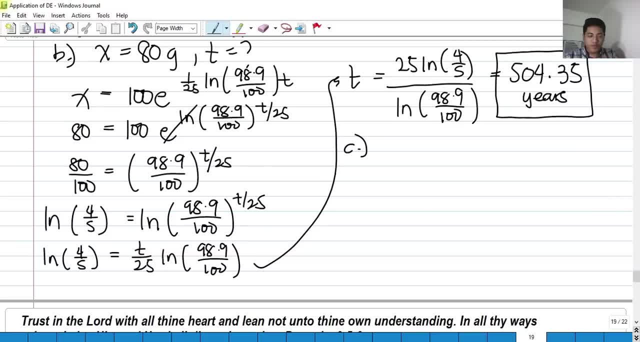 Okay, That is decomposed after 50 years. So our model equation is this: So I can get the amount of decomposed after 50 years. but that is not our answer. So we have 100.. 100 e raised to 1 over 25, Ln of 98.9 over 100. 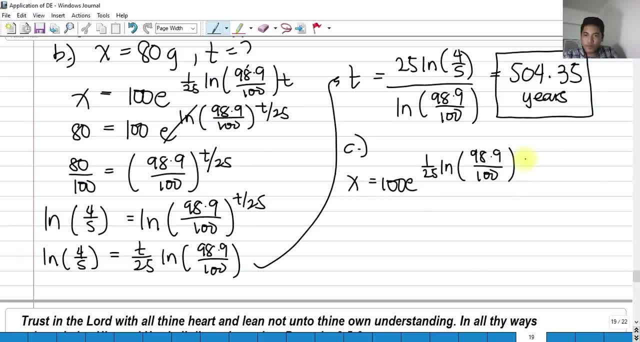 What is our time? Our time after 50 years? Okay, So, if we evaluate this, Okay, So you can also rewrite this as 100 e raised to 50 over 25.. Okay, Ln of 98.9 over 100.. 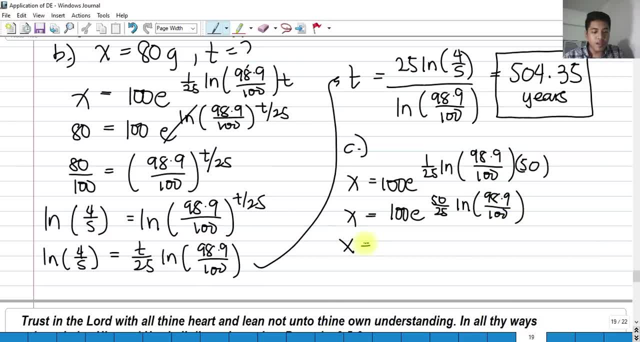 Okay, So if we get that, that is the amount remaining. That is not the answer. The problem is asking for us for the percentage amount decomposed. Okay, So we have 97.8 if I'm not mistaken, So 97.8 grams remaining after 50 years. 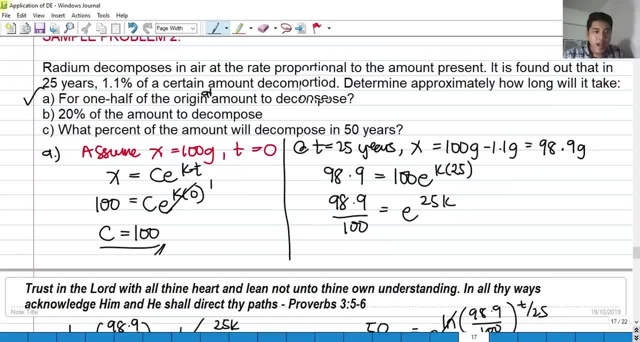 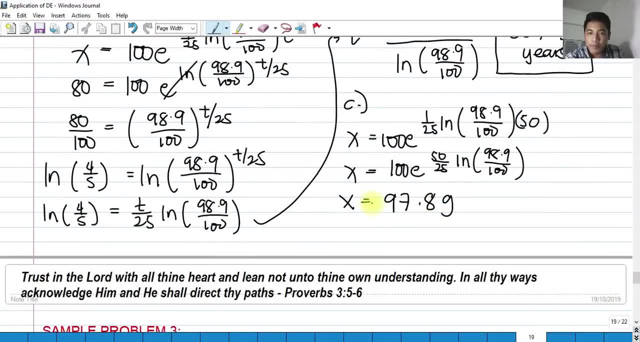 So that is not the answer, But because we are asked what percent of the amount will decompose in 50 years? What percent of the amount will decompose? This is the amount after 50 years. To find the percentage simply, our initial is 100 grams minus 97.8 grams. 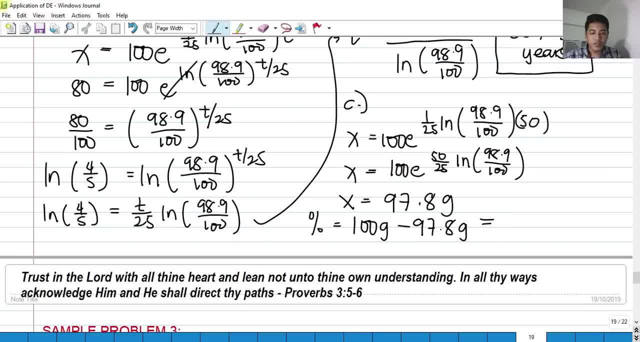 Okay, So that is the percentage decomposed after 50 years. Okay, So that is. Let's say this is 0.81.. Let's have it two decimal places. Let me just recheck this again. Okay, So we have 97.81.. 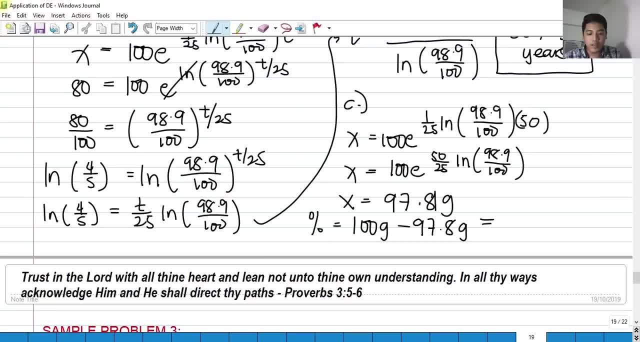 So 100 minus 97.81 is 2.19.. Okay, So percentage is 2.19%. Why did I say so? So the amount remaining after 50 years is 97.81.. Okay, So I'm going to get the percentage of this. 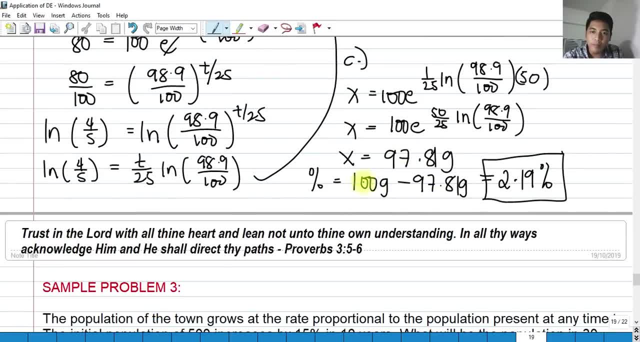 Okay, I'm going to minus, subtract the original, minus the amount remaining, And that is since we assume that we have 100 grams. Okay, So the percentage would now be the initial minus after 50 years, which is 2.19%. 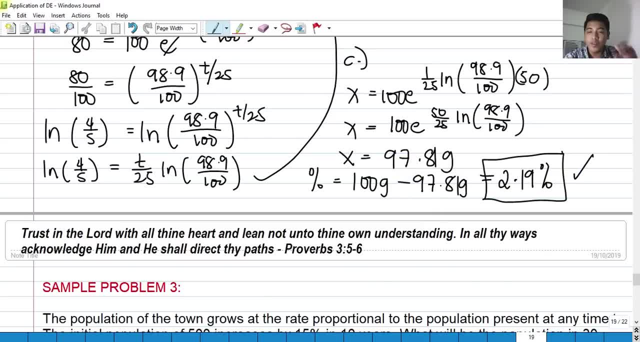 That is the amount decomposed: Percentage, amount of decomposed after 50 years. Okay, So another way to look at this is, if we minus this, 100 grams, minus 97.81, we'll be having 2.19 grams. 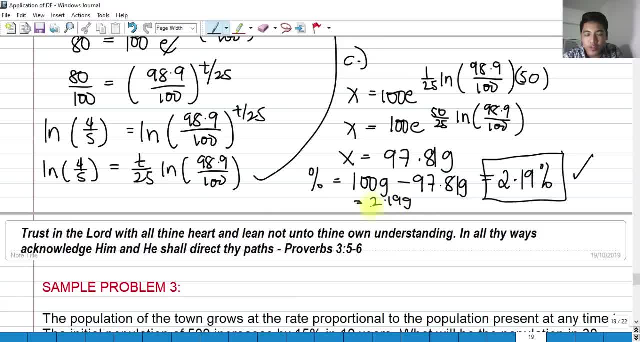 And if we are going to get the percentage of this based from the original amount of 100 grams, that should be 2.19 grams over 100 grams multiplied by 100.. As you can see, the 100 would Would cancel. 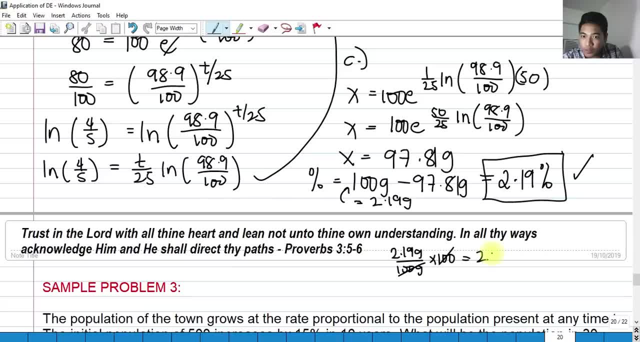 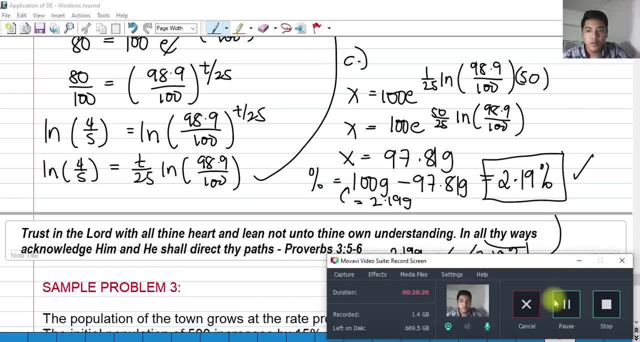 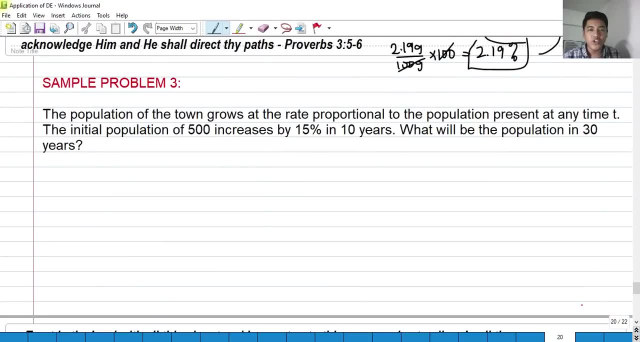 This is 100 because percentage. So we are left with 2.19%, which is still our answer here. Okay, So let's go now. Let's go now to our last problem. So our last problem: the population of the town grows at the rate proportional to the 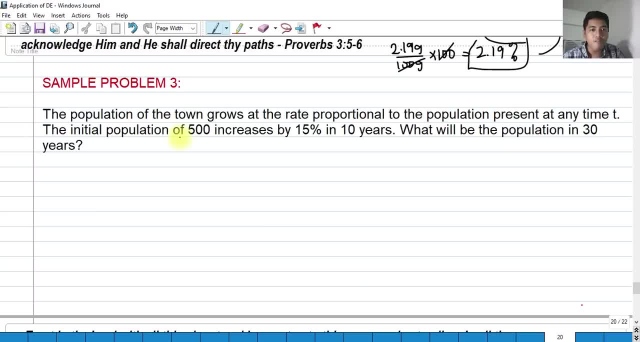 population present at any time. t- The initial population of 500.. Okay, That is our x. Increasing Increases by 15% in 10 years. What will be the population in 30 years? So this is a problem all about the loss of growth. 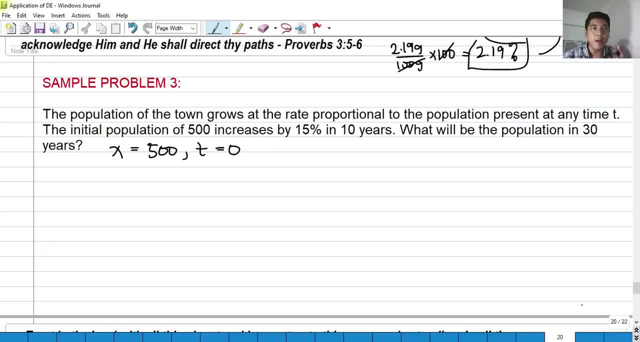 Okay. Population As population. as time goes by, the population is growing. Okay, So we have an initial value of 500. at time is equal to 0. Plugging it into our general equation of our DE, we have: 500 is equal to C, e raised to. 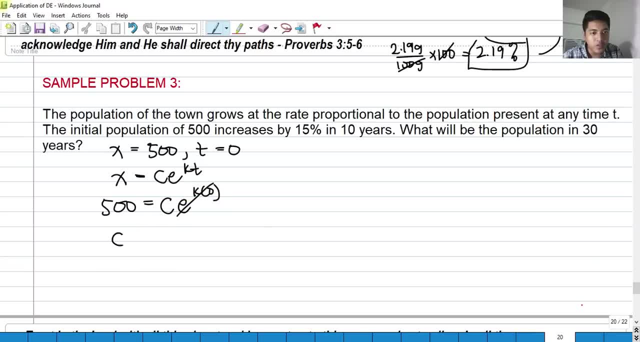 k times 0.. Okay, Of which this is only equal to 1.. So therefore, C is equal to 500.. Okay, And down to our second condition to find k, it says at time is equal to 10 years. 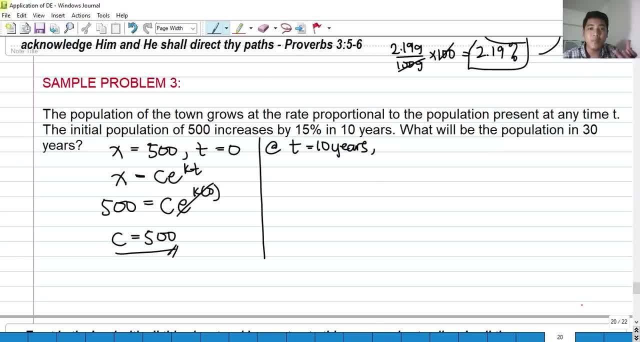 Okay, The population of that certain town increases by 15%, So our value for x should be 500 plus 0.15 times 500.. Okay, So, because it increases. So after 10 years it should increase by 15%. 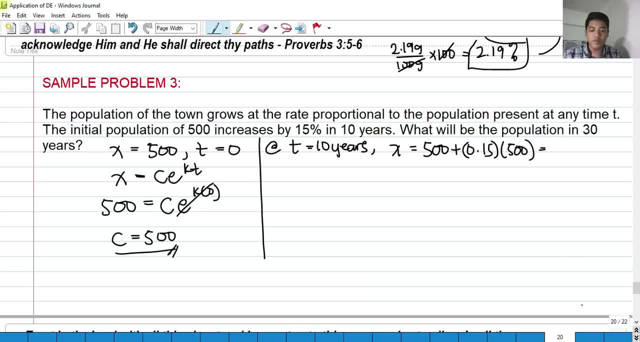 So 500 plus 0.15 times 500, that should be 575 populations. Okay, So plugging it in our equation again, this So we have 575 is equal now to 500, because that's the value of C e raised to k times. 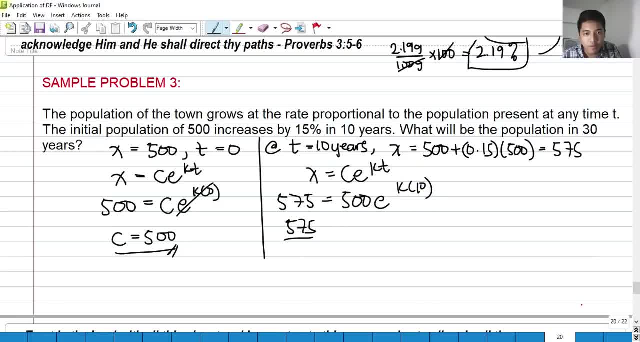 10. Okay, So 575 over 500 is equal to e raised to 10k If we ln or have the natural logarithm of both sides. so we have: ln of 575 over 500 is now equal to ln e raised to 10k, of which this should cancel. 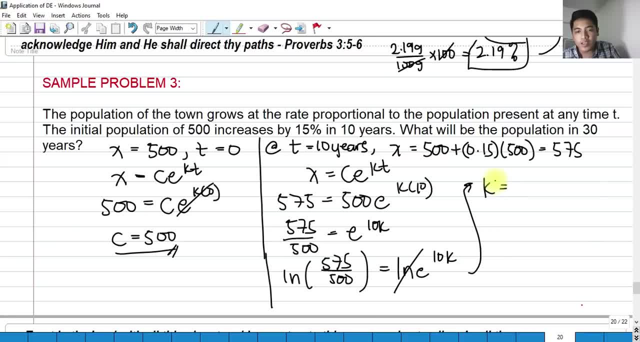 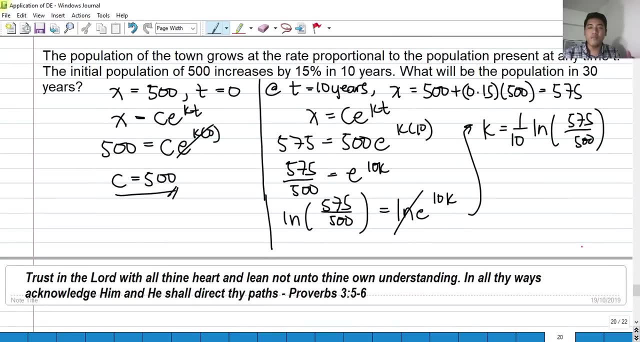 So we know what would be the value of k. The value of k should be: okay, 1 over 10.. Okay, 1 over 10 ln of 575 over 500.. Okay, So we now have the model for our equation, and our model for our equation is at the population. 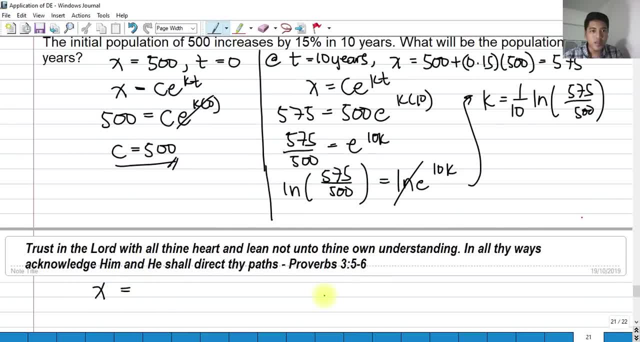 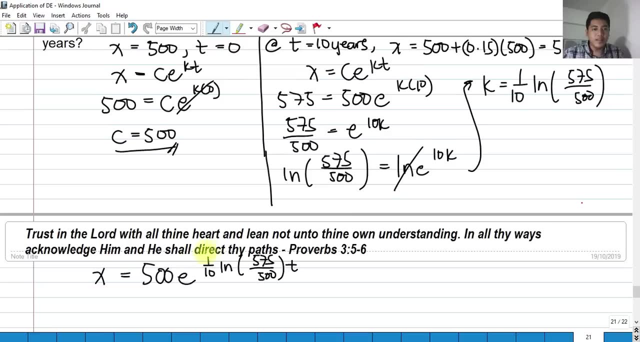 of time, any t or at any time t is should now be 500 e raised to k: 1 over 10, ln of 575 over 500 multiplied by t. Okay, And this can be also rewritten as x is equal to 500 e raised to t over 10, because this: